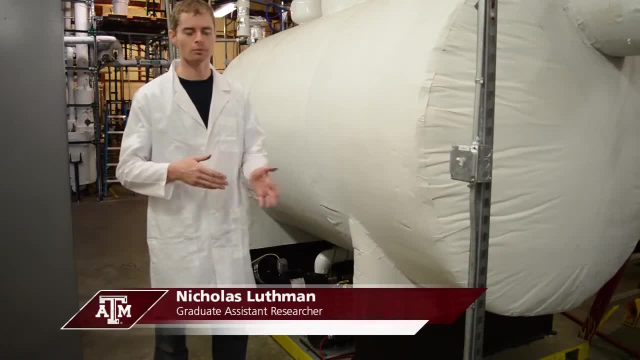 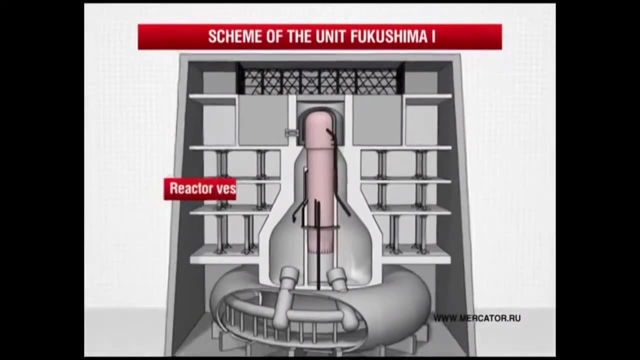 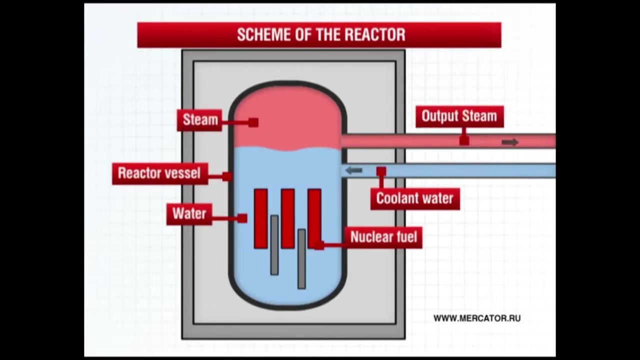 an analog to a reactor system that's used in many plants around the world, And our experiments here have in the past few years have involved injecting steam into a suppression chamber. So it's about filled halfway up with water and we inject steam into it And since it's 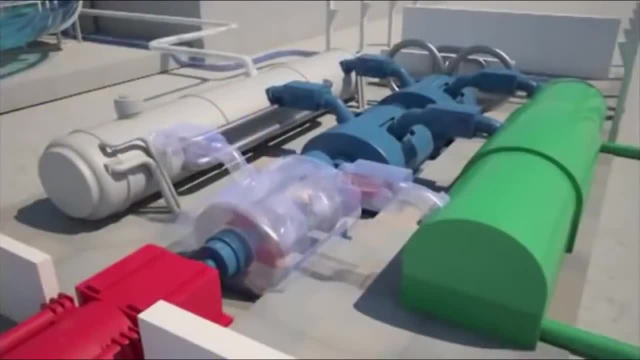 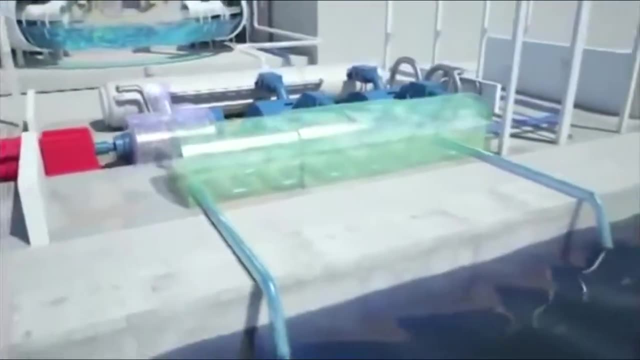 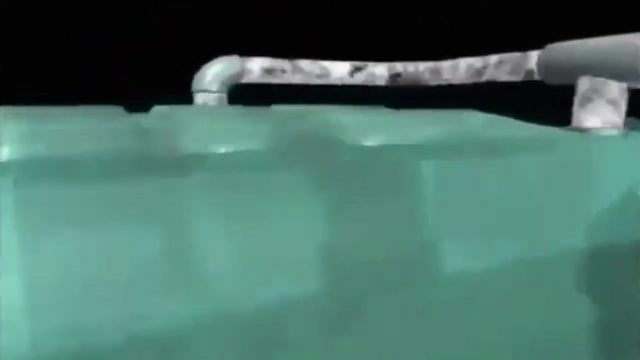 able to hold pressure, we're able to keep the pressure up. We're able to see how the temperature distribution is arranged as we insert steam through different flow regimes, And we found that it tends to stratify pretty well. Turbines are supposed to take in, operate well with gas, only They're not supposed to. 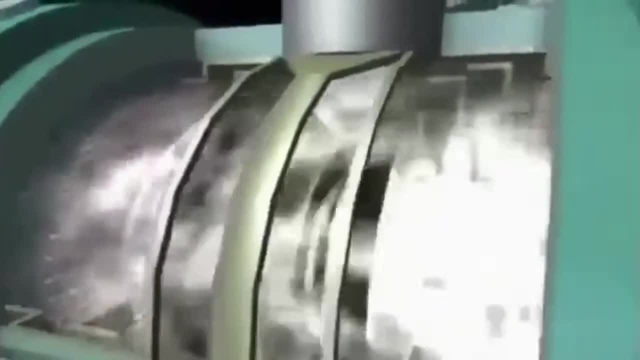 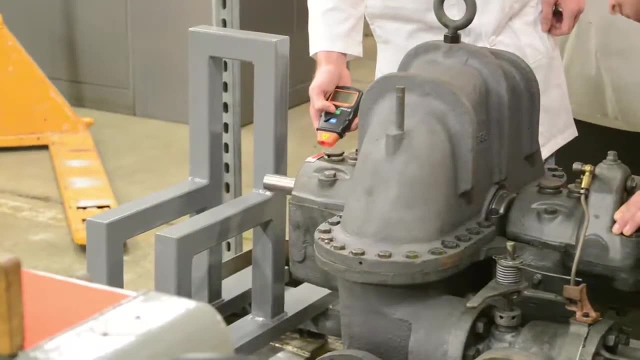 operate well when they ingest water, And we're fairly certain that at the Fukushima reactors they were ingesting water. The water level was high, became high, spilled out of the reactor pressure vessel Into the turbine, and yet the turbine performed fine, even though it was taking in water. and 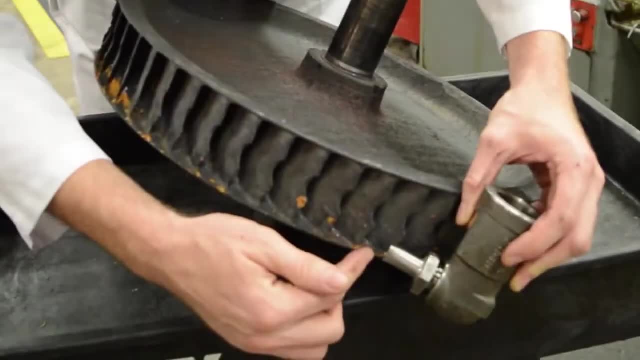 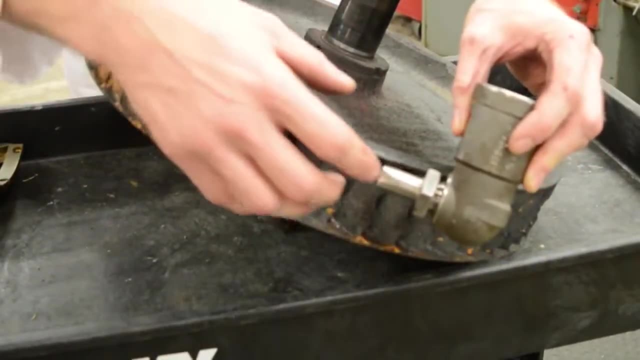 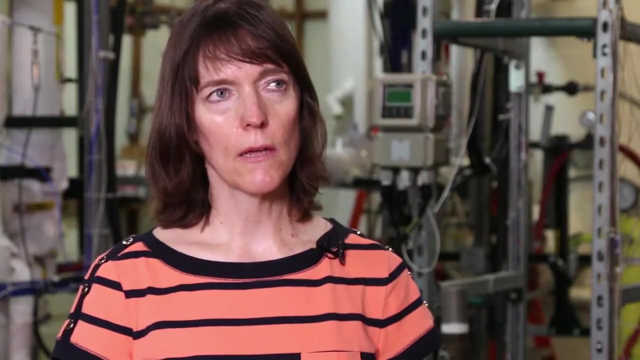 steam. So we'll be doing some testing here where we inject water and steam into the turbine and get a better handle on how it performs with this two-phase steam-water mixture going into it. We've been learning a lot about how the water recirculates in the system and when. 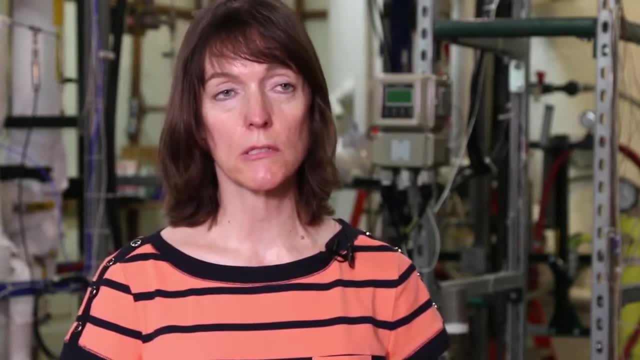 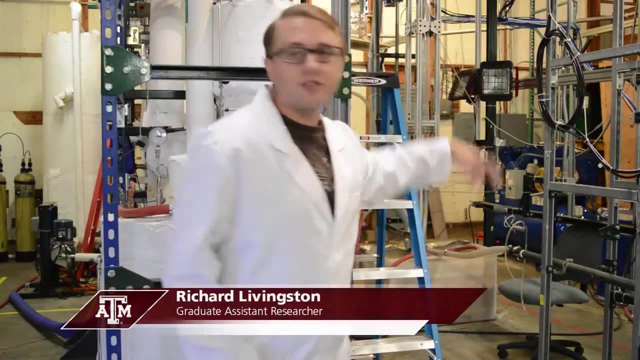 we're approaching thermal temperature limits that won't let the system operate any longer. So what we do is we initially inject water from the top of the test section. That actually forms an annular film around the actual test section. Once the annular film is established, 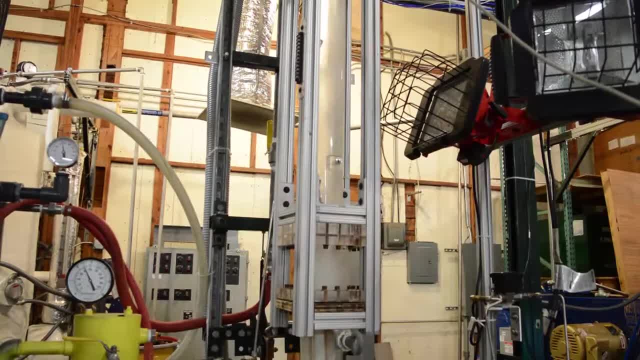 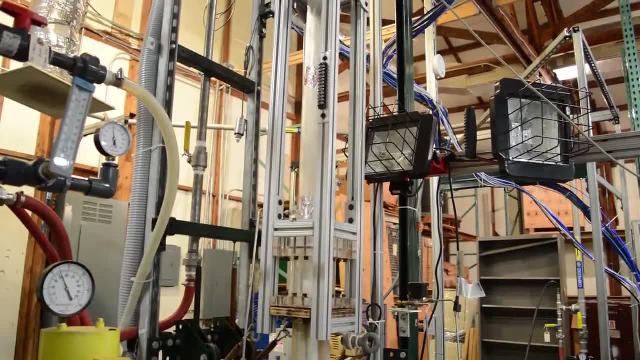 we then actually inject air from right here into the bottom of the test section, And once that air actually reaches at critical velocity, reversal ends up occurring in the actual water. So one thing that's happened is that one way to cool off a reactor during shutdown is actually injecting water into one of the steam exit channels, And that's actually what we do when we inject water into the reactor. So we actually inject water from the top of the steam exit section. That's what we do, And once the water goes into the reactor, we actually inject air. 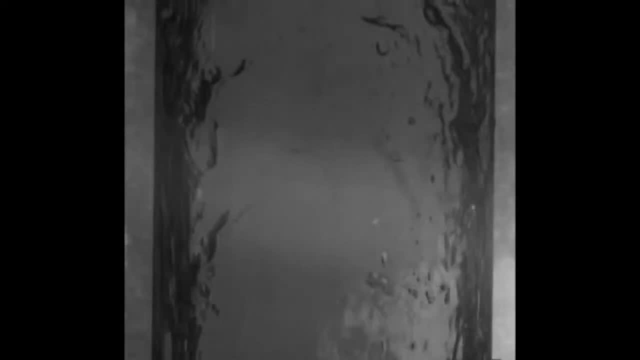 what we're looking at is some of the issues that arise is, if that steam is going too fast, it actually stops water from getting into the reactor core and cooling core.